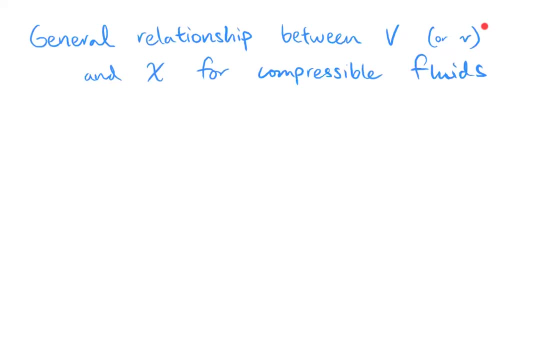 and just like earlier in the course we went over this sort of generalized stoichiometric table, here we'll go over the, this sort of general relationship between volume and conversion. So I'll first draw this as if it were a flow system. But really these two situations, at least for this concept, are not going to be so. 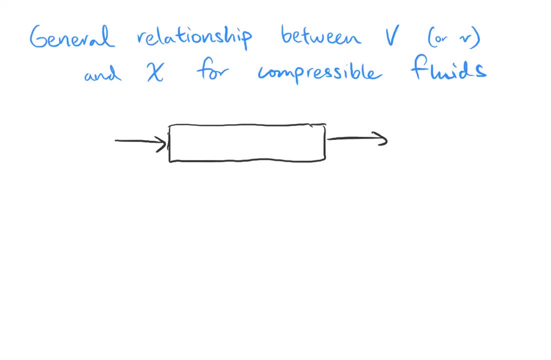 different. So we have something coming in, some components coming in, and some components leaving. Let's say, we have then our volumetric flow rate in and a volumetric flow rate out, And so we have a situation where, because our fluids are compressible, 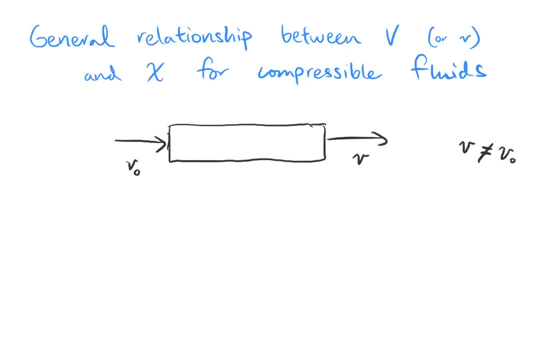 and these two terms are not equal- And so we might have all kinds of components here, like A0, B. we might also have an inert species. Let's go ahead and write what this with this reaction would look like. So there's going to be a reaction here. 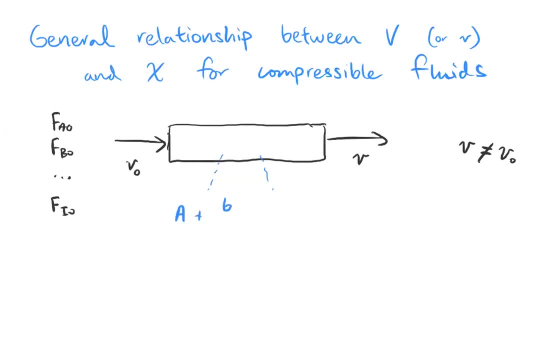 and I want to write it with stoichiometric coefficients So that we can see, at least this is all on a basis normalized to the stoichiometric coefficient of A. so we have A plus little b over little a times b. Those are the reactants. 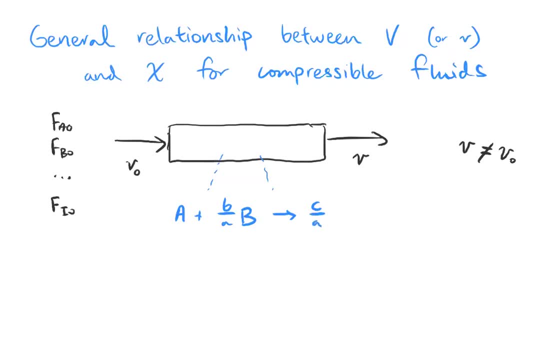 yielding products C and D of this stoichiometry of C over A times C plus D over A times D. okay, And we will let that go and see you guys in the next lecture. So thanks again for taking time out to watch other videos. See ya later. 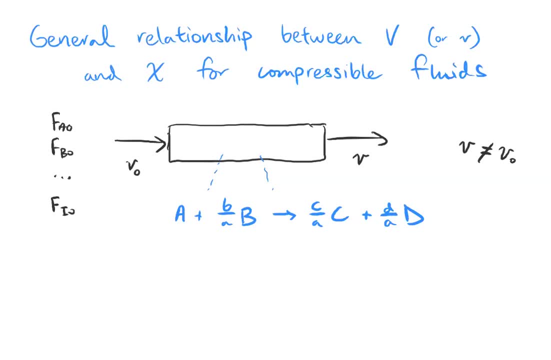 with this before to ultimately come up with a stoichiometric table. Now here I want to kind of point out that you know, generally when we're interested in the mole fraction of species, we know it's the number of moles of that species over the the number of total moles, and it could also be the molar flow rate of. 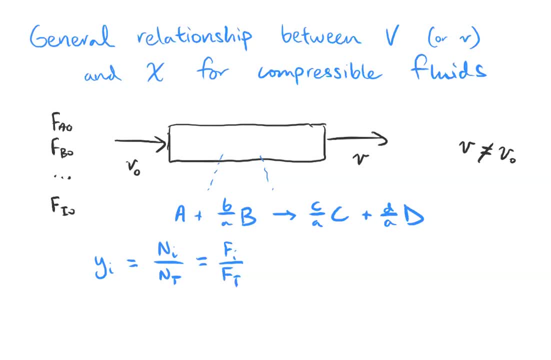 that species or the total molar flow rate. but, either way, something that we know that we want is kind of this understanding of: well, how much does the the, the total number of moles or the total molar flow rate when we make our sample? the total number of moles or the total molar flow rate when we make our 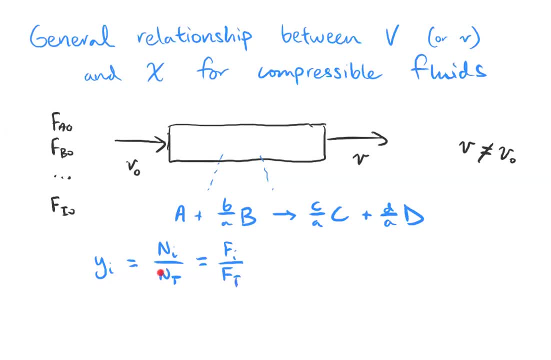 stoichiometric table. we're largely interested in what that number is and also how conversion relates to these terms. So the sort of shortcut to recognize here is that you have your number of moles at any given time is equal to, and this is: the total number of moles at any given time is equal to the. 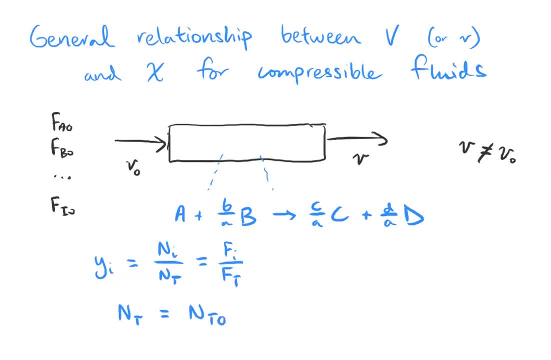 the total number of moles that you started with, plus- and I'm going to use this lowercase delta symbol here- multiplied by your number of moles, initially of, in this case, since everything is is normalized- A, which you would treat as your limiting reactant. it's the number of moles of your 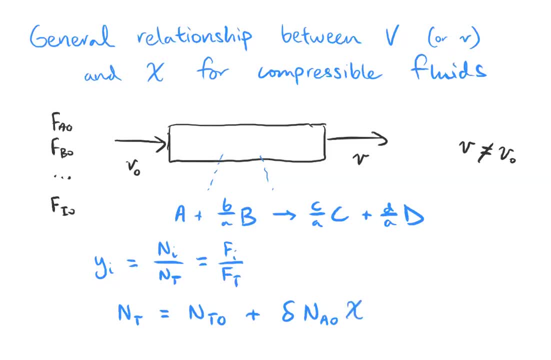 limiting reactant times your conversion. Okay. so then the real question is then: what is this delta term? Because if we knew that, we could very quickly get to plugging in this term and then perhaps we could also recognize what we always do with mole fraction. 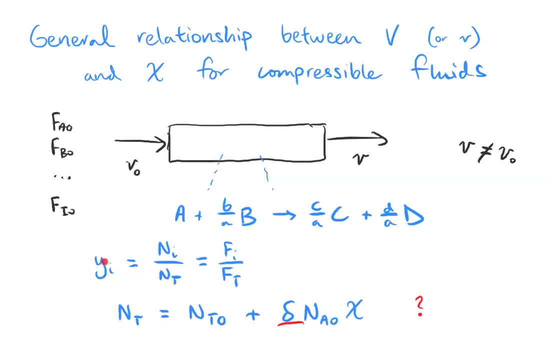 since we essentially just use the ideal gas law to figure out how we can relate concentration to these terms. And so what I want to explain here- I'll try to fit it on the same page- is that delta, as you'd find from your stoichiometric table, is, is going to be. 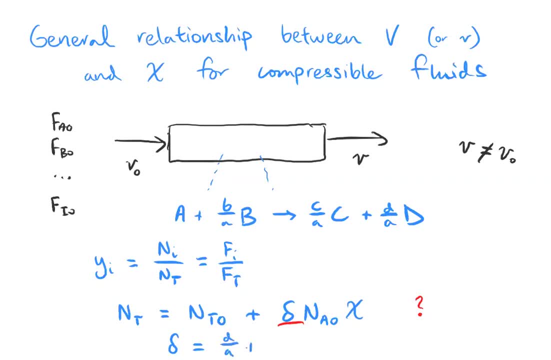 just D over A plus C over A minus B over A minus 1.. And what it essentially is just change color. it's the change in the in total number of moles over the mole of A reacted. Okay, so what can we then do? 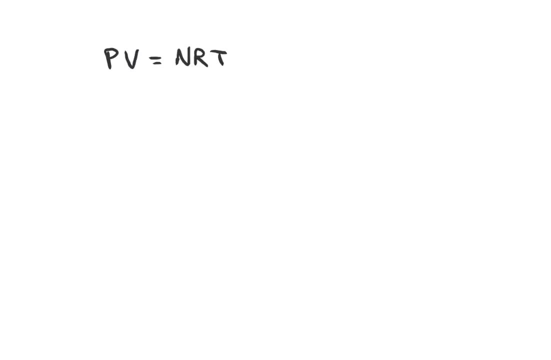 with this. Well, if you take this equation and you think about the total number of moles, So I'll just say this is n total. This is an equation of state that is valid at any time, So it must also be valid when you started. So if you just kind of imagine the initial set of conditions, 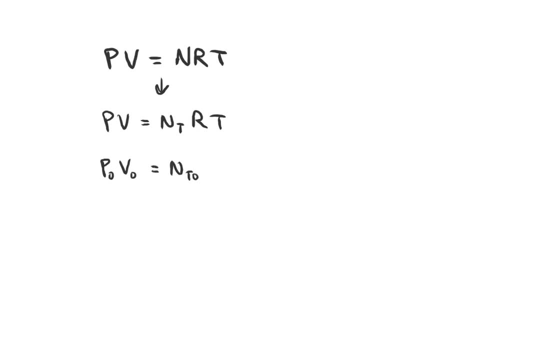 you know, at some point you had an initial total number of moles and you had that at a given pressure and volume and similarly an initial temperature. So you could imagine comparing these two and actually performing division to be able to get this relationship when you isolate for just volume. 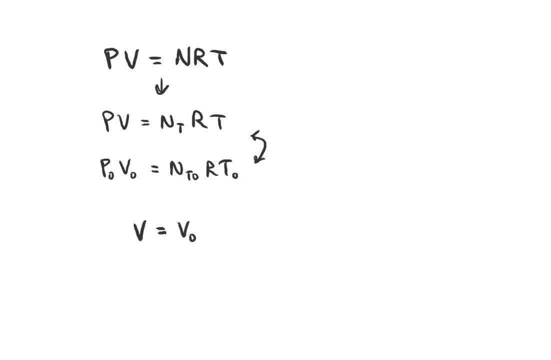 The volume that you would have at any given time is going to be equal to the volume that you started with. times the initial pressure over whatever pressure you're at now. times the temperature you're at now over the initial temperature. And again, this is just coming from the fact that you know temperature and pressure are on different. 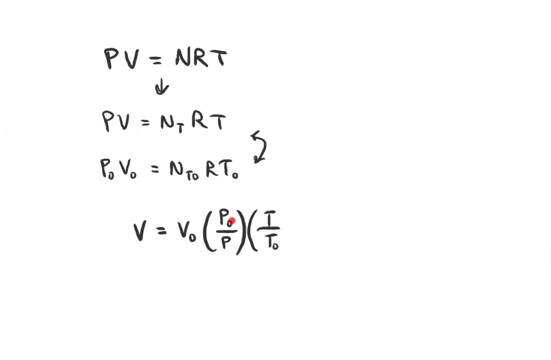 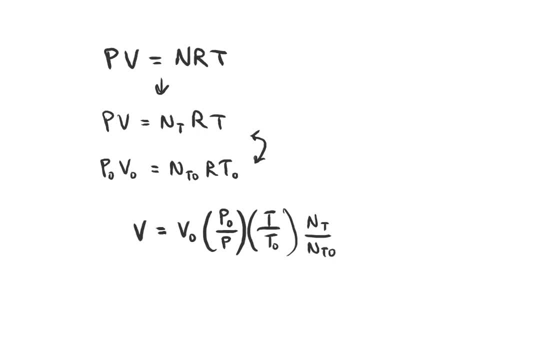 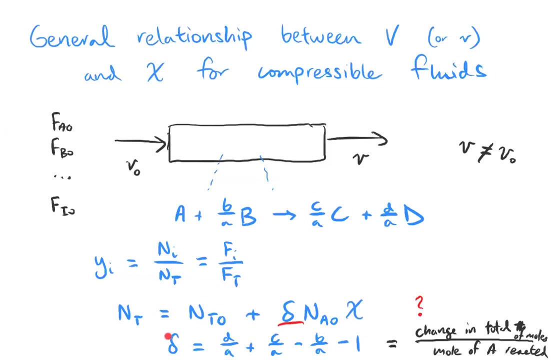 Okay, And so we can already see where there's sort of an opportunity to be able to just thinking about on the previous page- utilize this sort of relationship of how the total number of moles is influenced by the is related by the conversion. 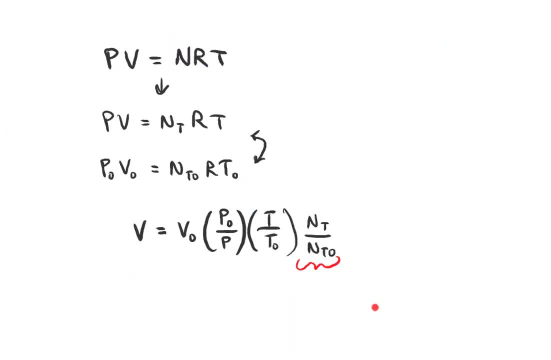 So if we take that and sort of put it back here, we have. you know, Nt over NtO equals one plus that mole fraction, since we have everything on a basis of A. And so if we just take that and and and sort of put it back here, we have. you know, Nt over NtO equals one plus that mole fraction, since we have everything on a basis of A. 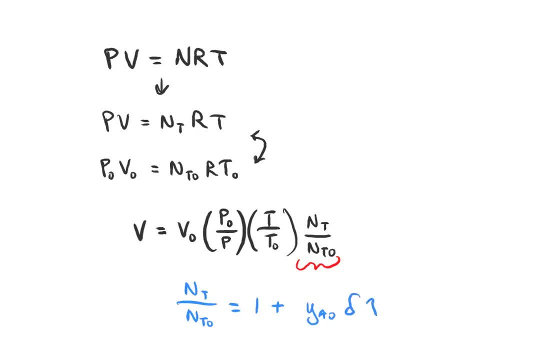 times delta times the conversion, and so what that just tells us overall is- let's see if I can still fit it here- is that v, the volume at any given time is equal to what it started off as, and then you have this pressure and you have temperature, and now you have just one plus the mole fraction. 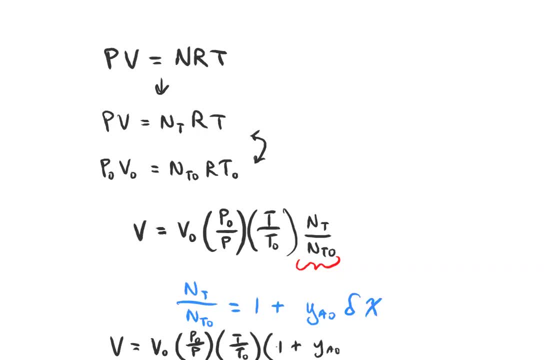 a initially times Delta attempts conversion. okay, and so this didn't get rid of your need to still figure out the mole fraction of a initially, but it does greatly simplify the kind of approach and stoichiometric table that you might want to prepare, because now you don't, you don't need any. 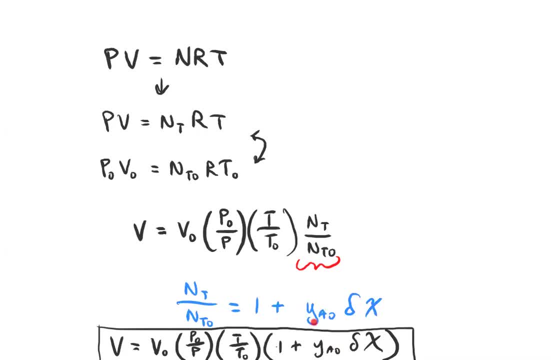 of the terms of the final, the final composition. you just need to know what your initial mole fraction was. similarly, you're in most of your problems. you're not gonna have pressure and temperature also changed, changing, For example, like Robert's problem 4-3, it's isobaric and it's isothermal. So 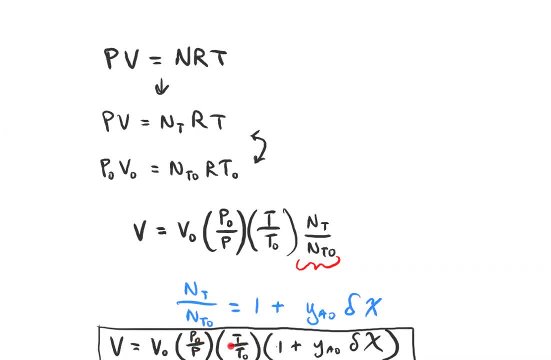 this just immediately shortcuts. you know these terms become one, and then you just have this clean and quick relationship between what the volume is at any given time and what it was originally. And lastly, maybe this is a good place for me to note that if you're